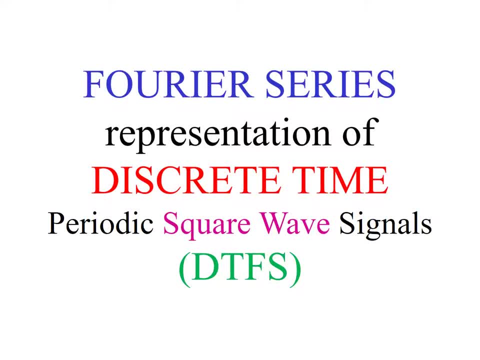 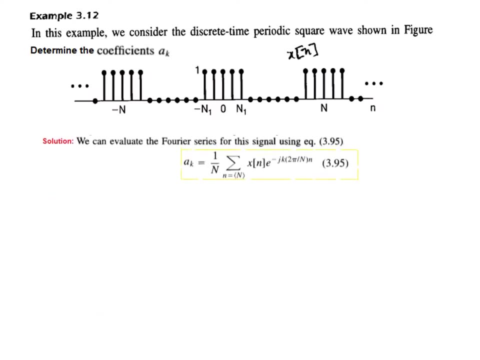 Bismillahirrahmanirrahim, This is the second part of four year series discrete time periodic signal and this will just deal with the square wave signal. So this is the square wave signal, It's a periodic signal and we have to determine the coefficients a, k. 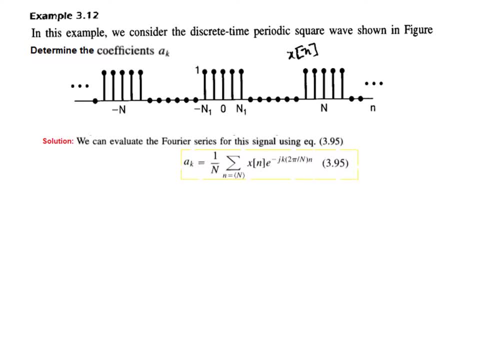 So we have learned earlier in the previous video that the one of the methods of finding coefficients is given by this formula: a, k, one over n, which is the time period. xn, the signal value. e raised to the power minus j, two pi over n and multiply by small n. 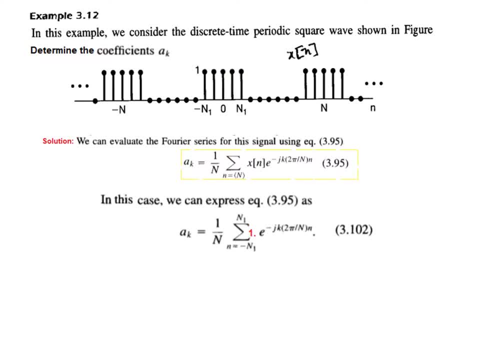 Now, since the magnitude is one, therefore for xn we can write one. Also here the limit was n, But because so n could be like from here to up to this point. So any recurring point, or from here up to this point, or from here up to this point. 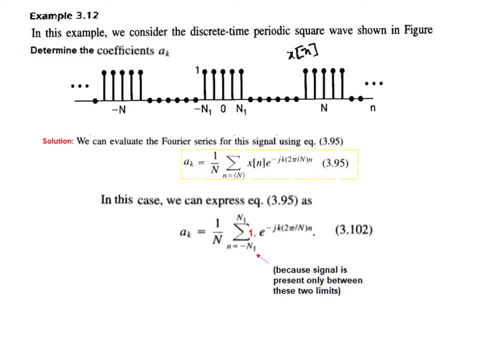 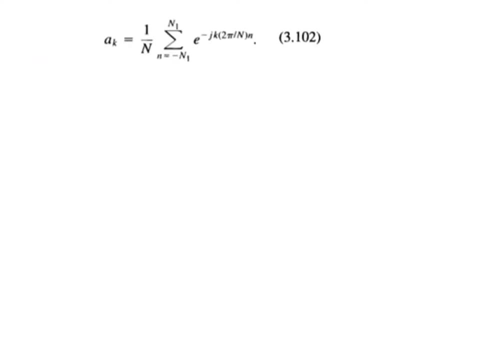 So, but in this case, since the signal is only present between minus n one and plus n one, Therefore we'll put these two limits. So we were here. now We know the formula of a summation When x is not integral to one. 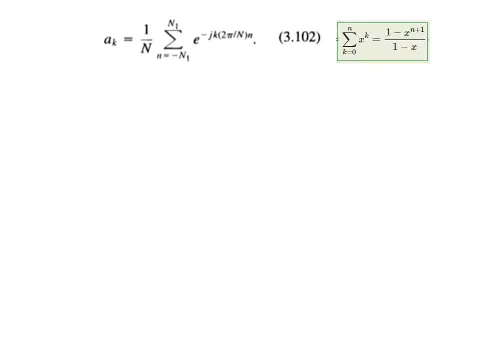 This is the formula that we use. That means we would like that this should be zero. to match with this, k equals zero, And for this we'll have to take help of another variable, And for this we'll have to take help of another variable. 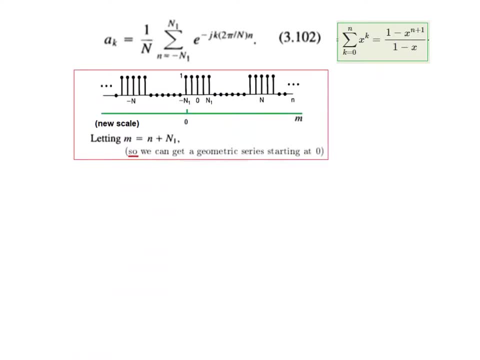 And for this we'll have to take help of another variable. So we take help of a variable m Which starts from zero at n minus one, Or mathematically we can say that this new variable m is equal to n plus n minus one. 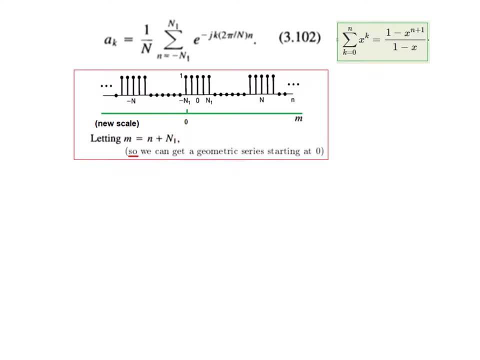 Remember, when we put this equal to zero, then n becomes equal to minus n one. So n minus one or zero is at n minus one. So n minus one or zero is at n minus one. Okay, So now if we try to find the two limits, 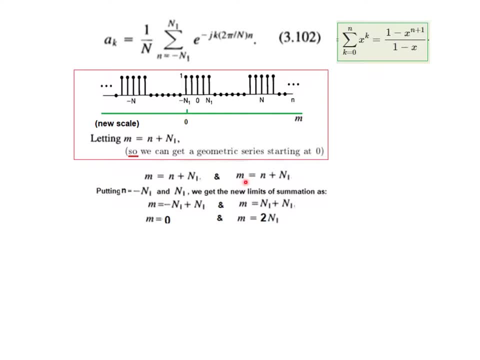 So m is n plus n one, M is n plus n one. And then we put the two values for small n equals minus n one And plus n one. So minus n one if you put here, it becomes zero, And plus n one if you put here. 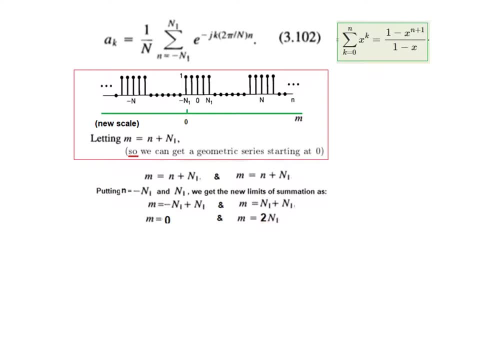 And plus n one. if you put here 1, if you put here, it becomes 2 and 1. so the limits now is from 0 to 2 and 1. okay, so this is the new limit. rest of the things remain same and now we can open. 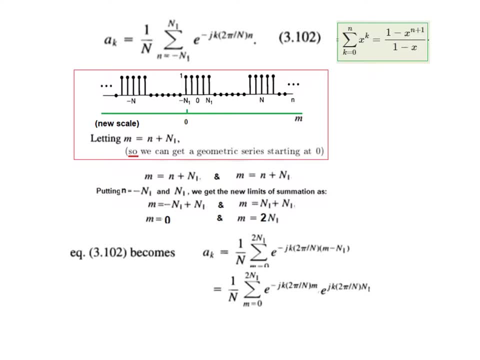 this bracket, we can break it into two parts and, as you know, that plus sign or minus sign is represented by the multiplication of the two signals for E JK, E JK 2 pi n, 2 pi n M and again another E JK, 2 pi n minus n 1. so this: 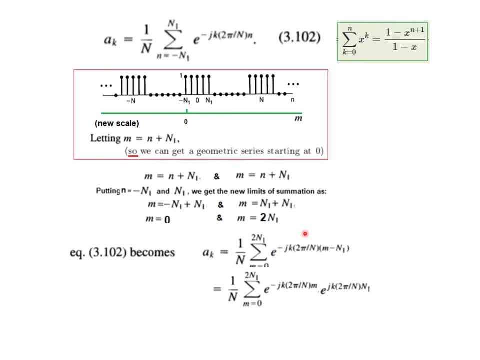 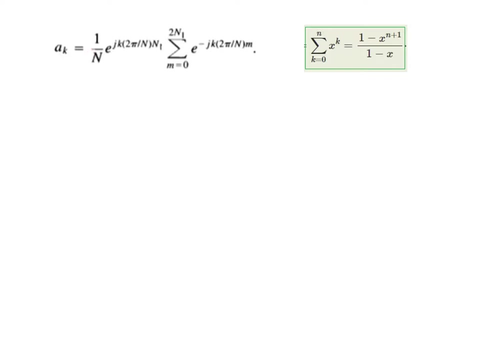 and there's a minus outside, so this one become plus and the first one will become minus sign. and since this term does not depend on M, therefore this is a constant term, so we take this out and the only term containing M remains within this summation. so you adhere, we're taking out the constant term outside this summation. 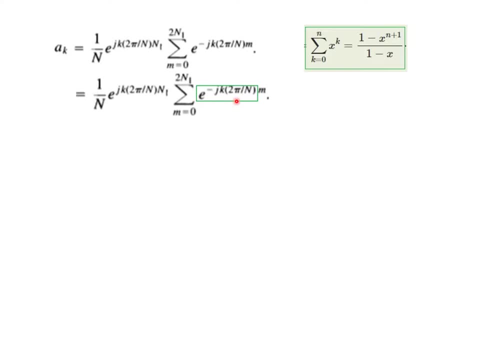 and now you can see that this water is multiplied with the variable'm. so this is the variable them, which is wearing from m 0 to 2 and 1. and now compare this. if you compare this with the signal, this whole thing can be called as X, and M has the two limits here, K has the two limits. 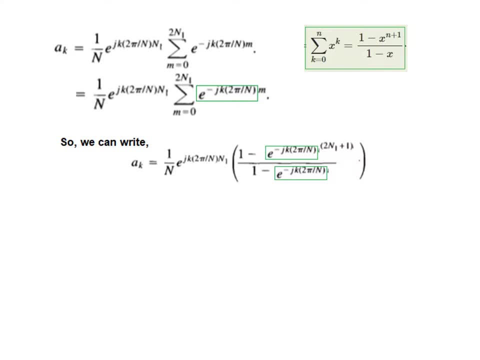 so 1 minus X. so we write 1 minus this whole thing in the box. that is our X, n plus 1. so the maximum limit n plus 1. in our case maximum limit is 2 and 1. so we will write 2 and 1 plus 1 and in the denominator it is 1 minus X, so it is 1. 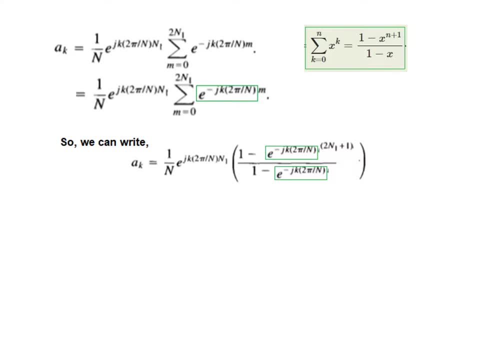 minus the box. and now we just little bit of manipulation to now this: this whole thing is multiplying. so E, JK, 2 PI multiplied by 2 and 1 divided by n, this is what we get. bottom remains same. and now we'll use a trick. see, if we had 1 minus e, power minus X, we could write 1. 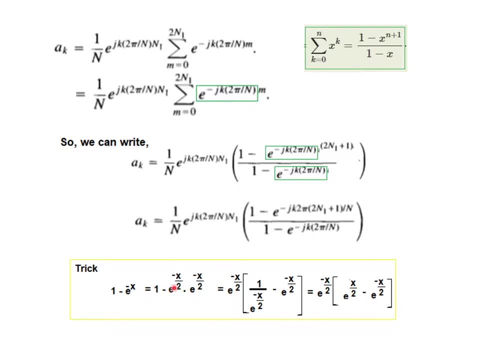 minus e and divide the X into two parts, so X over 2, X over 2. and if you solve this, e raised to the power, minus X over 2, minus X over 2 will be minus X. so we have divided in 10 to 2 parts. and now if we take common e, minus. 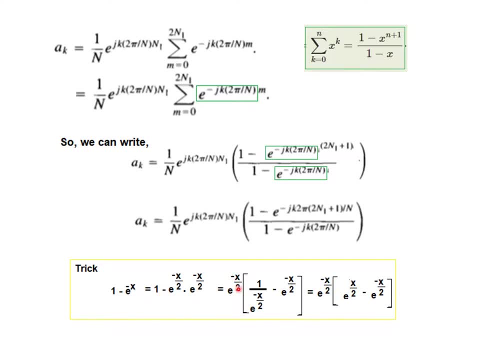 X take a common from this. so e minus X by 2 we take common. so here it will be 1 divided by e dash to the power minus X over 2, and here e minus X over 2 get one of the e minus X over 2 will get cancelled. 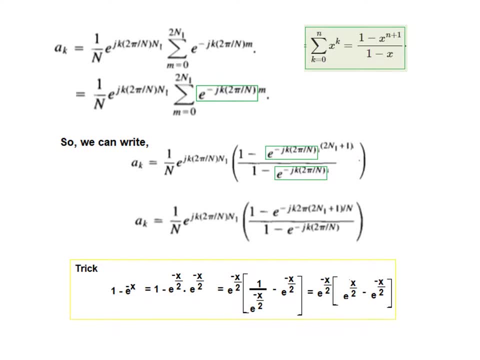 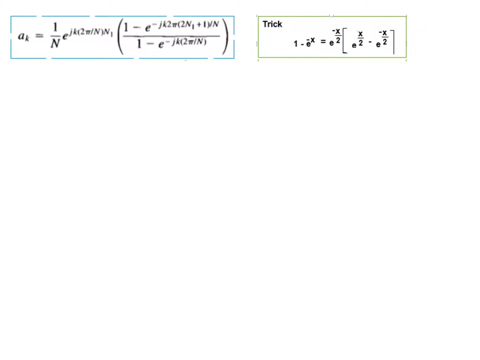 so it is minus e, X over 2 and now 1 over he is to the power. minus X over 2 can be written as e plus x over 2 power. this is our final answer. same technique will apply here. okay, so this was the signal that we had, and they say the: 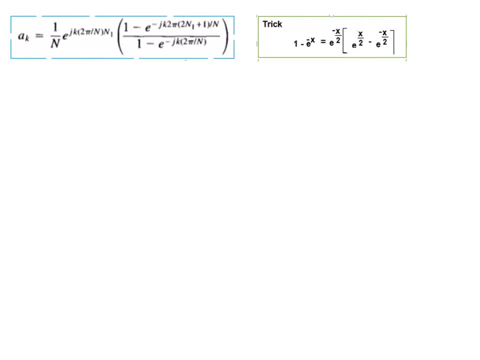 technique that we would apply here now. we will have to write the equation now, as I told you before, the equation we are going to follow, so let's do it very carefully. you can see the first part. we are just doing it in two parts. we're taking the numerator and the denominator separately, so 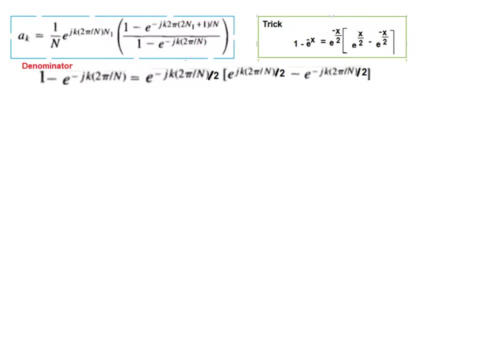 first. this looks easy, so we'll do the denominator first: 1 minus ej k 2 pi n dividing into two parts, and take a common. just follow this, exactly same. so e minus j k 2 pi n divided by 2, we take common, and then we have e plus j k part, and then we have minus e minus j k part divided by 2, both. 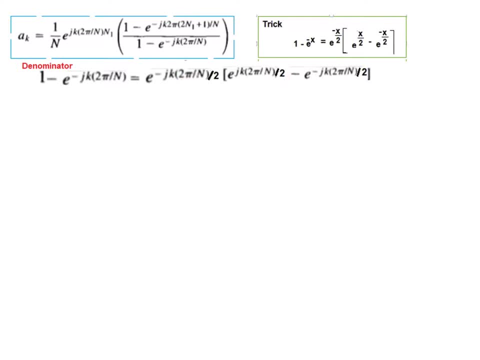 exactly same copy, just putting the values, and by further simplifying we can take to inside. so it is 2 pi over 2 n, 2 pi over 2 n and 2 pi over 2 n and 2 to cancel. so here it will become e minus, j k pi over n. e plus, j k pi over n. minus, e minus. 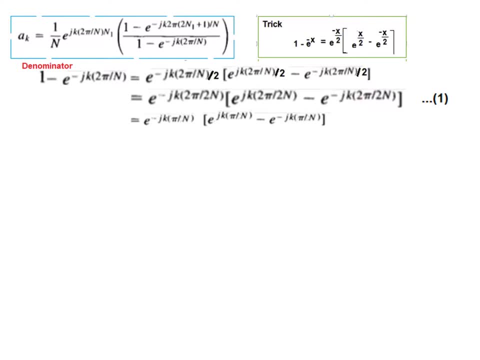 j, k pi over n, so all the twos get cancelled. okay, and now we again take help of euler's formula for sine. it is ej theta minus ej theta, same as it is here. so just this part will be sine theta multiplied by 2j. so we can say that: 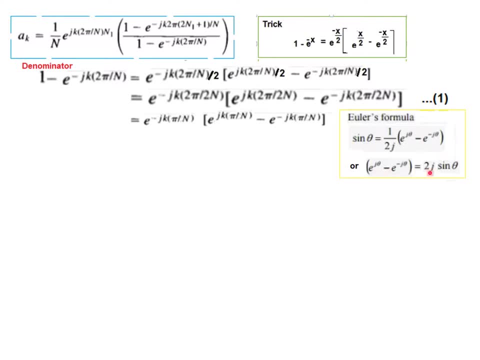 ej theta minus. ej minus theta is 2j sine theta. so we will also put 2j sine, whatever is the value of the theta here. so this becomes e minus j k. pi. n first part, its same inside, is replaced by 2j sine pi k over n. now we come to the numerator part, same technique. 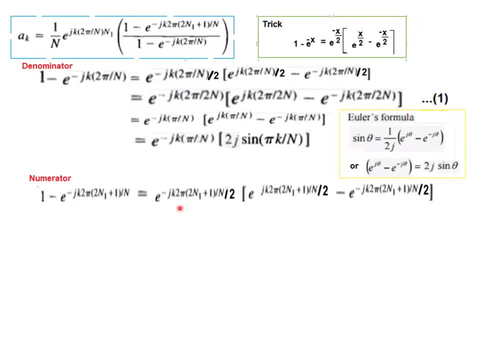 this FAR from k and that is divided into two parts, taking common exactly replica. and here also we have replaced the internal in the bracket terms with the sign theta sign terms. okay, so this was the original. will now replace the denominator and the numerator with the new values in terms of a sign, so the 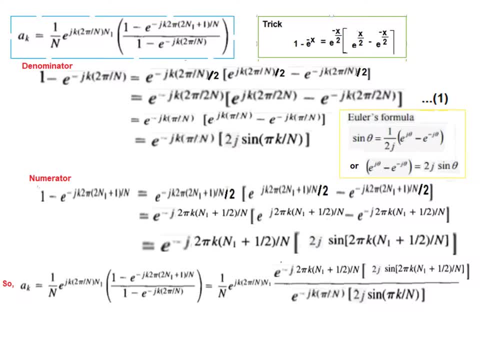 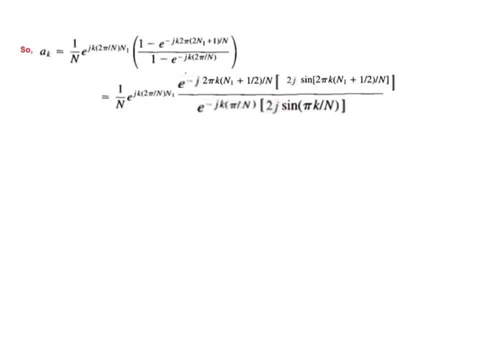 constant remains here, and then this part comes from the numerator and this comes at the denominator. okay, so by putting the value of numerator and denominator, we now get this complete term here and now. if you take this term out here and then the numerator and denominator remains as shown here and this can be now broken. 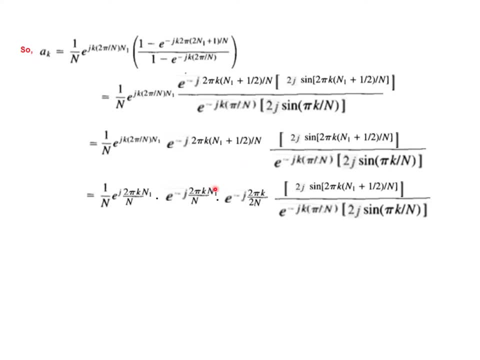 down. this is a plus. so we break it down into two parts: 2 pi K and 12. pi K and 1 divided by and, and this is to multiply by 1 come 1. so is pi K, 2, pi k n divided by geomAKER Fusion. 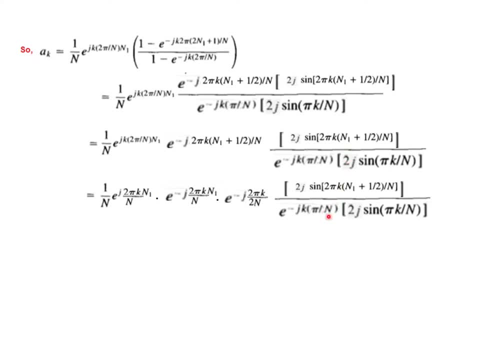 and this term remains. sembs will divide x plus u addition 1 x half fala in G. Divide it later. It's not divided now, Just multiply. And now we divide everything by 2 wherever it is possible. So first of all, we see that these two are the same terms. This is a negative sign and this is a positive sign. 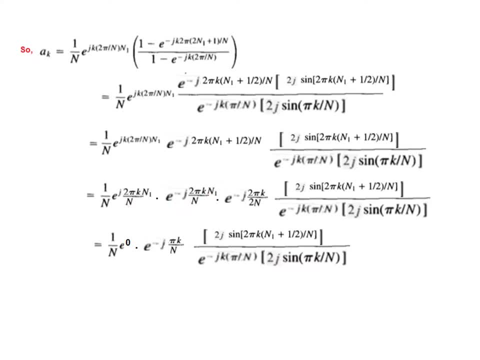 So when you add the powers it will become 0. This term we divide by 2.. So it is e minus j, pi by kn And the remaining terms remains as it is. So finally, e raised to the power, 0 becomes 1.. So this is the term left, So 1n, e, j, pi, kn and the two terms of the denominator and numerator. 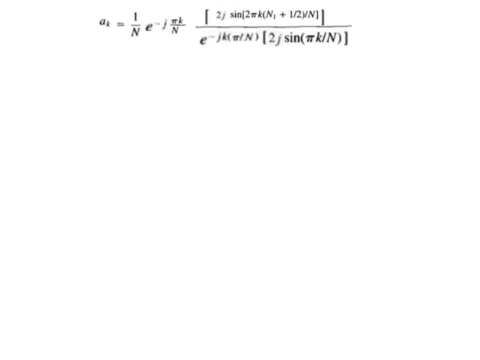 So we were here. And now, if we cancel these two terms, same terms, So our equation will become 1 over n and the numerator and this denominator term. And now if you multiply by 2, then it will become 2n plus 1.. 2n1 plus 1.. So it will become like this. 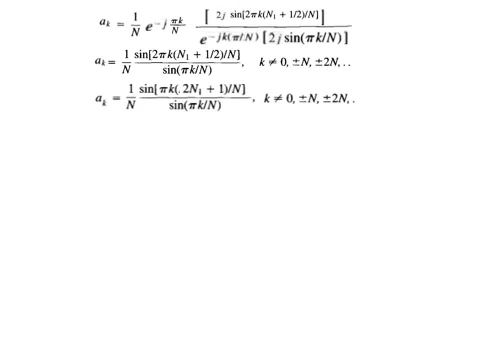 So this is the equation for finding coefficient. a k when k is not is equal to 0, or not is equal to n, or not is equal to 2n, etc. Now to find the value of a k, the coefficient when k is equal to 0. 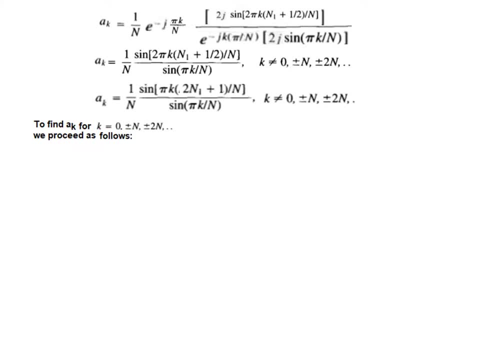 or it is equal to n or 2n. we proceed from the equation 1 0- 3 that we got earlier, where we converted the variable n into m. So this was the equation that we had gotten there. Now, if you put, k is equal to 0.. 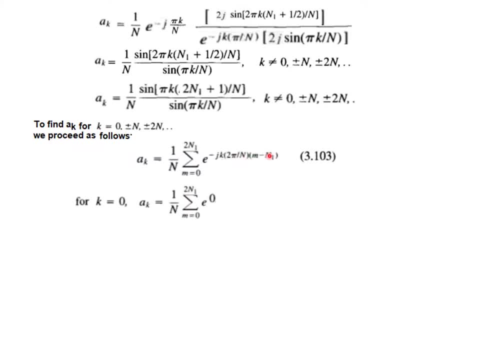 So k equals 0. This means that this whole term becomes 0.. So e raised to the power 0 is equal to 1.. And this with the help of e raised to the power 0 becomes 1.. And by using the geometric formula, geometric series formula. 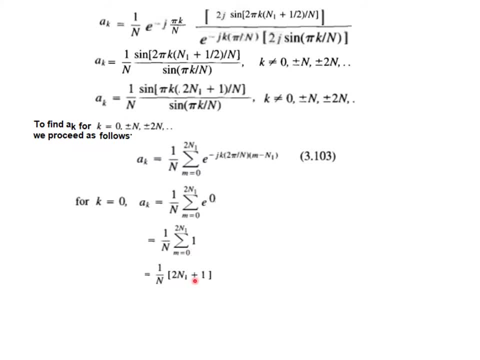 this can be written as 2 and 1 plus 1.. So a k can be written as 2 and 1 plus 1 divided by this n. This is when k is equal to 0 or plus minus n, or plus minus 2.. So these two equations are now with. 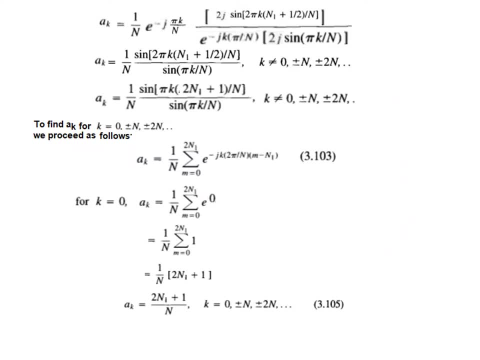 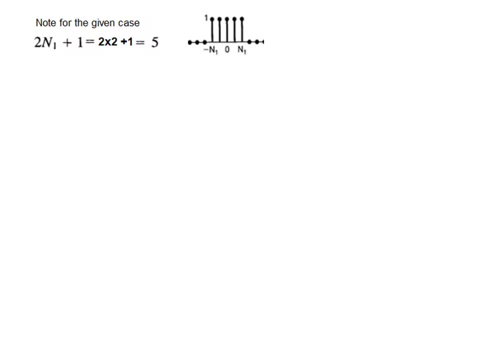 us and using these we will solve the problem further. Okay, for the given question: 2 and 1.. So this is n 1. So it is 0, 1, 2.. So 2.. 2 multiply by 2 plus 1, 5, or you can just. 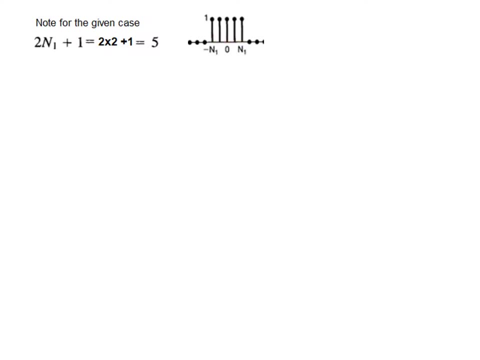 count. There are 5 values, 5 positions, And we will just solve one problem for n, or the time period equal to 10.. So these were the two formulas that we will be using First, for a 0, we will use this: 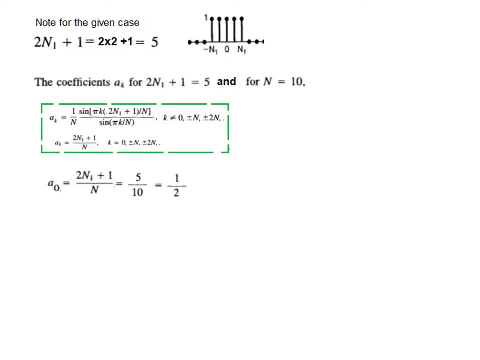 formula k: 0.. So 2 and 1 plus 1 divided by n, This one is 5 from here and n is in the 10. so 1 over 2 is the value for E naught for all other values till K is equal to. 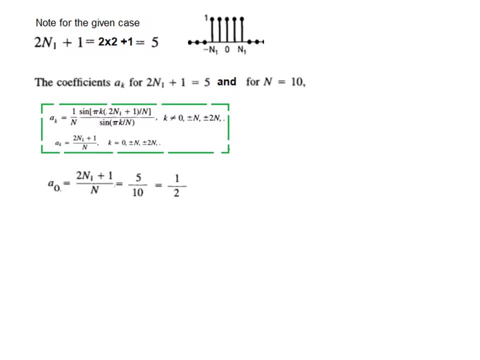 9. we will be using this formula. okay, so this is the formula, for K is equal to 1. we put K is equal to 1, so this term was given by numerator 1 and denominator zero. point three was multiplied by 1 over N, or 1 over 10, so the value for a 1 is 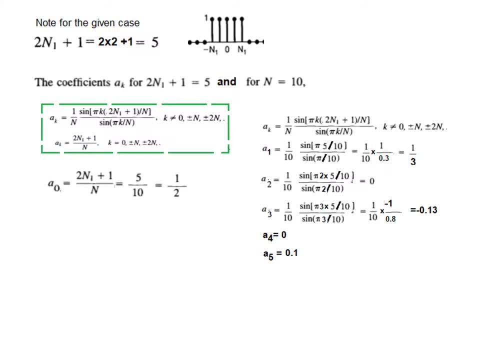 1 over 3. now for A, 2,, K is equal to 2, and nat2g, followed by sum of 2 into y and to 10. so this will become sine pi 10. 10 cancels and this will become sine 2 pi over 10. so this: 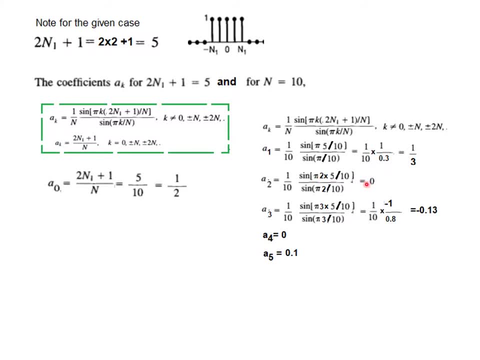 sine, pi, as we know, is 0 and therefore a2 is equal to 0. coming on to a3, put k is equal to 3 and we get a relation. use your calculators. this one is minus 1 and the denominator is equal to 0.8 x 1 over 10, so we get a value of minus 0.13 and a4 again will be 0, like we had. 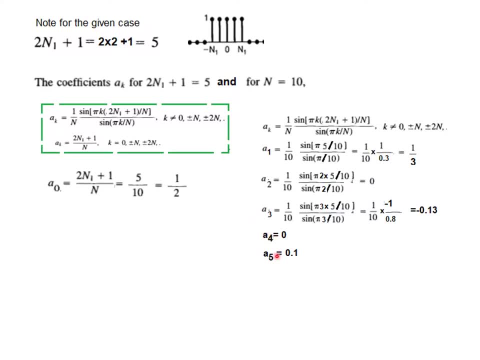 a2- here say a4- will be 0 and I hope you can calculate for a5. its value will come to be 0.15. just put 5. 5 here says 25 divided by 2, so sine 2.5 pi, and this will be half. so anyway, calculate the value. it will come to be 0, 1, okay, 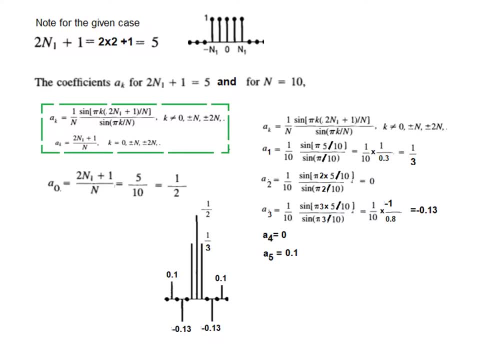 so the plot should look like: this is 0 half, this is 0, then 1 over 3, 1 over 3 on both sides for A1 and the a minus one, then a 2 is 0, so a2 is 0, A minus 2 is 0 and a 3 is 0.13 minus. so this is 0.13 minus a 3 and a. 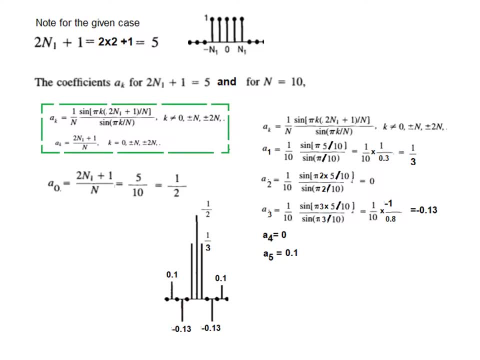 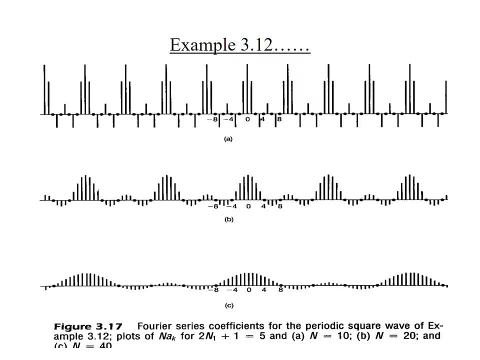 minus 3, a 4 is 0 and a 5 0.1. so 0.1 and this is a complete picture. for this n is equal to 10. if you increase the value to, n is equal to 20. you should get a plot like: 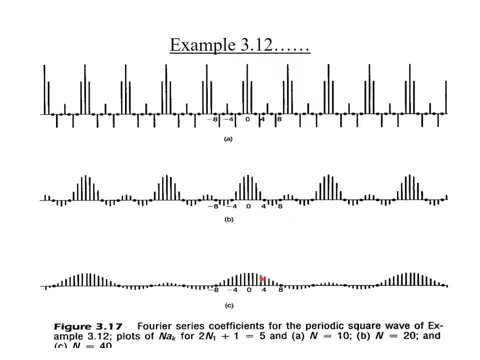 this and for n is equal to 40, you will get a plot like this: I hope this gives you some idea as to how to solve a square wave problem.